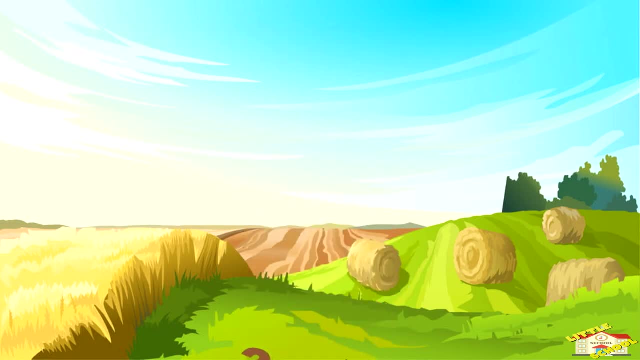 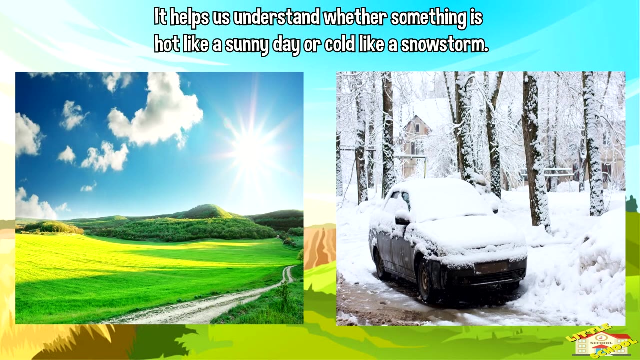 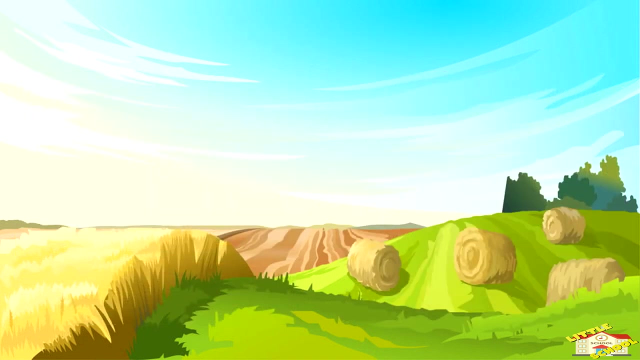 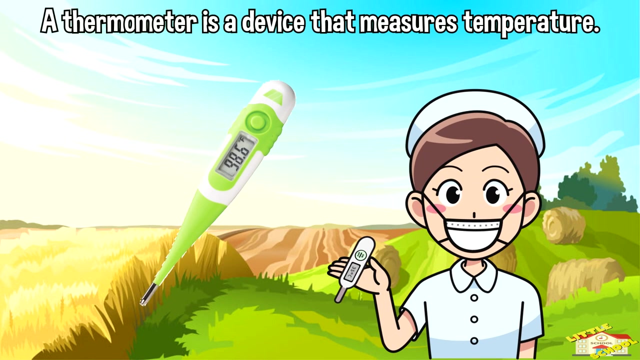 What is temperature? Temperature tells us how hot or cold something is. It helps us understand whether something is hot like a sunny day or cold like a snowstorm. We can measure temperature using a special tool called a thermometer. What is a thermometer? A thermometer is a device that measures temperature. 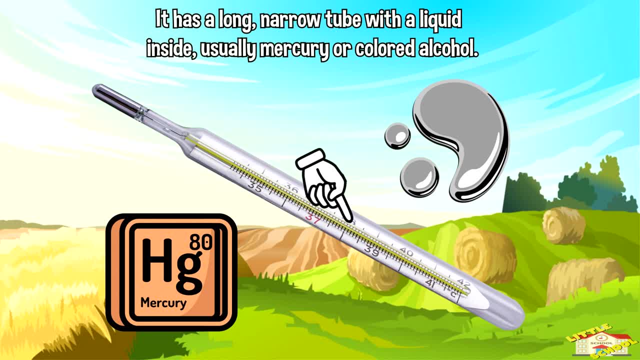 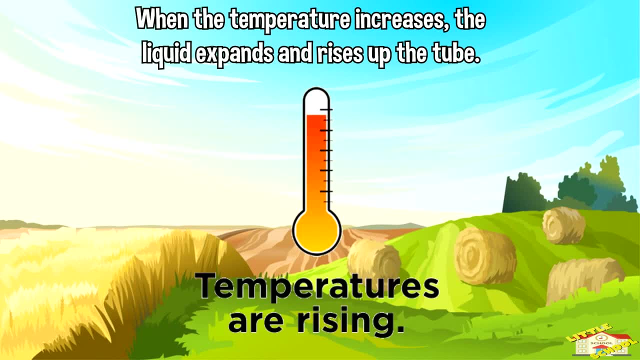 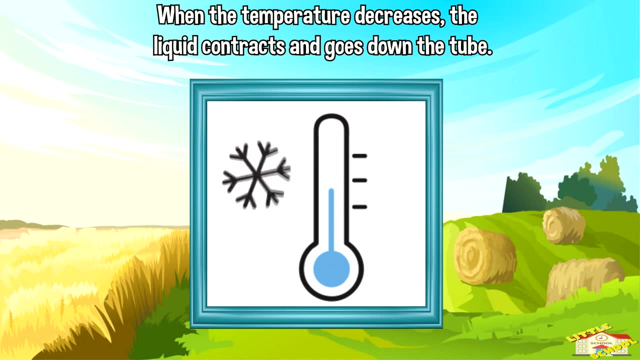 It has a long, narrow tube with a liquid inside, usually mercury or colored alcohol. When the temperature increases, the liquid expands and rises up the tube. When the temperature decreases, the liquid contracts and goes down the tube. When the temperature decreases, the liquid contracts and goes down the tube. 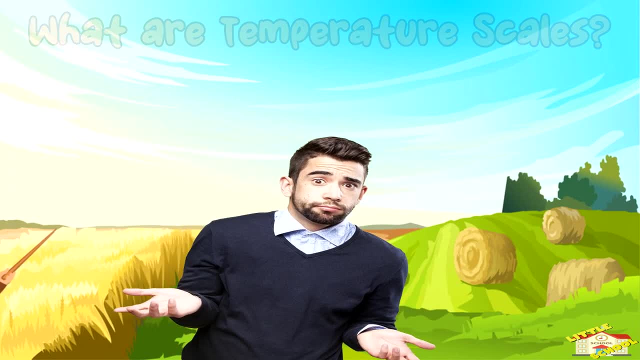 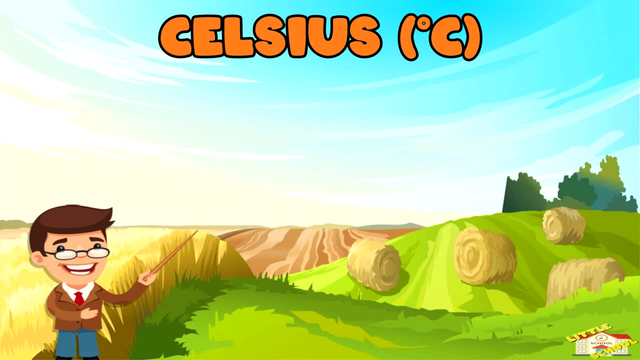 What are temperature scales? Temperature is usually measured using different scales. At a temperature scale, a temperature meter is measured in님 Celsius. distance speed: H1 temperature is 100% Plus th. In most countries temperature is measured in degrees Celsius. 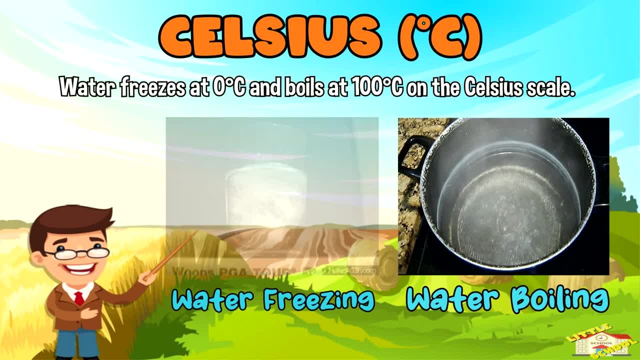 In other approaches, like cold water, we underwater temperature measuring for cold water. Water freezes at zero Celsius and boils at hundred Celsius Or just in the sameар At a temperature scale. water freezes and boils stress easier than freezing Like a stretching thermometerのは. 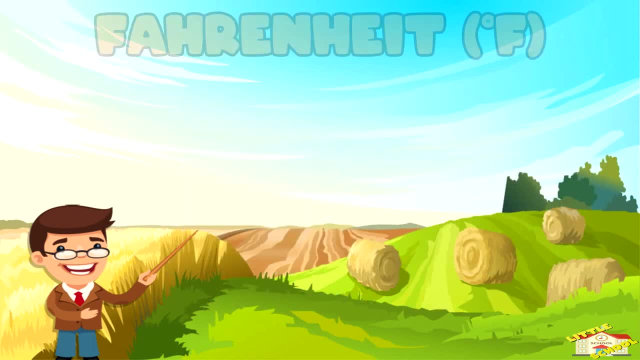 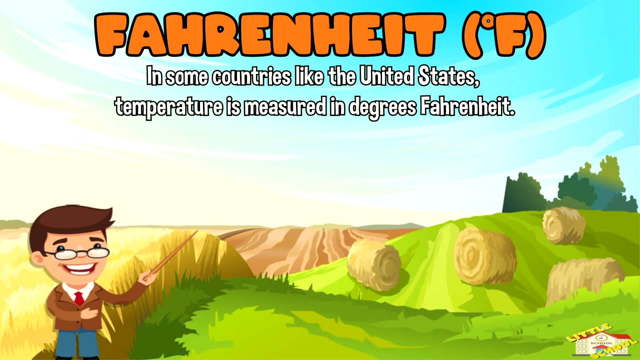 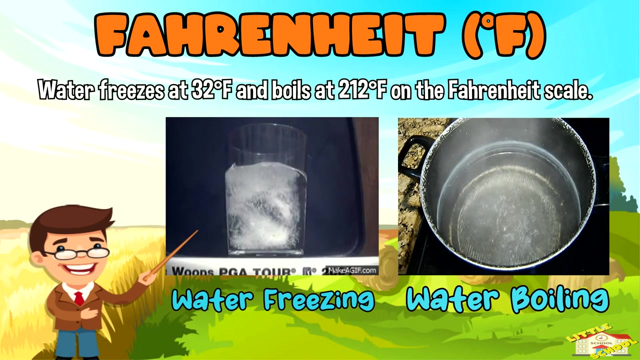 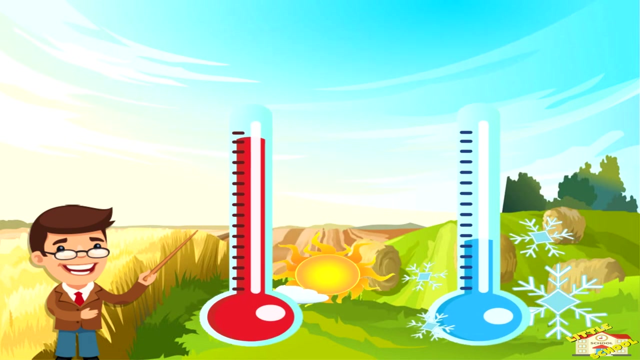 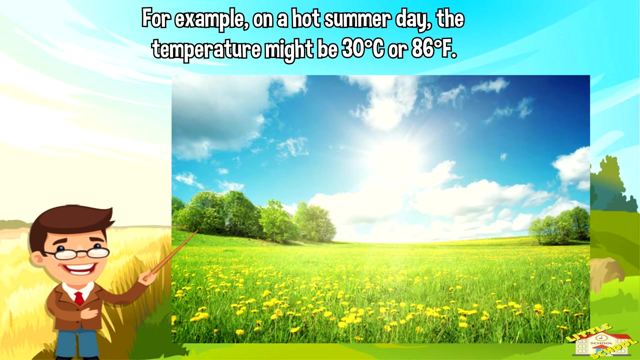 the Celsius scale Fahrenheit. In some countries, like the United States, temperature is measured in degrees Fahrenheit. Water freezes at 32 Fahrenheit and boils at 212 Fahrenheit. on the Fahrenheit scale Hot and cold: When something is hot it means it has a high temperature. For example, on a hot 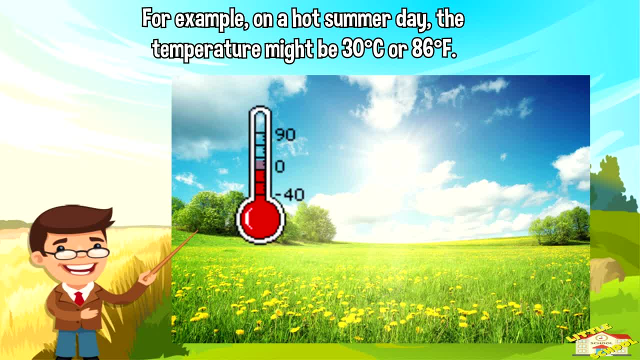 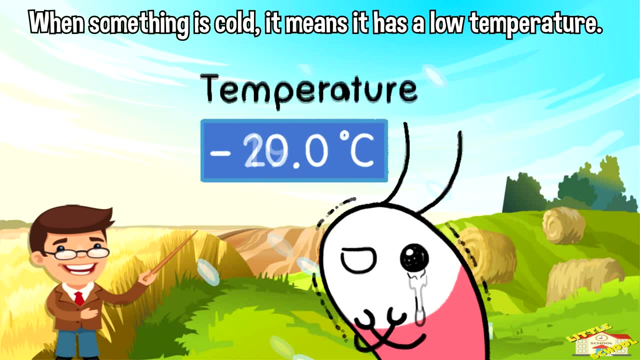 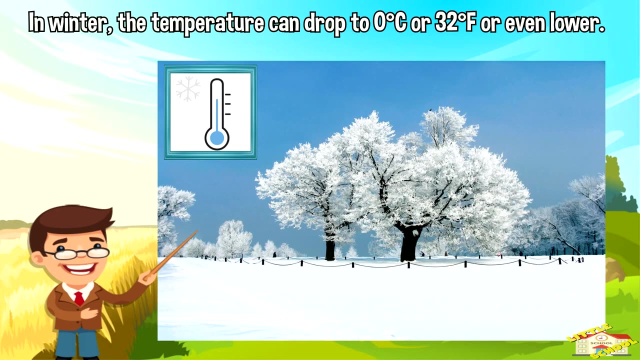 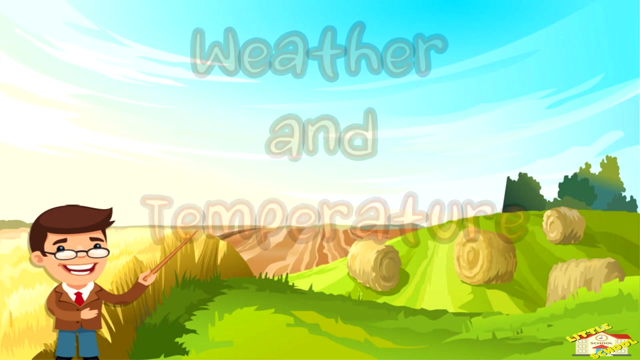 summer day, the temperature might be 30 Celsius or 86 Fahrenheit. When something is cold, it means it has a low temperature. In winter, the temperature can drop to zero Celsius or 32 Fahrenheit or even lower. Weather and temperature Temperature is closely related to weather. When the sun is shining, it warms.